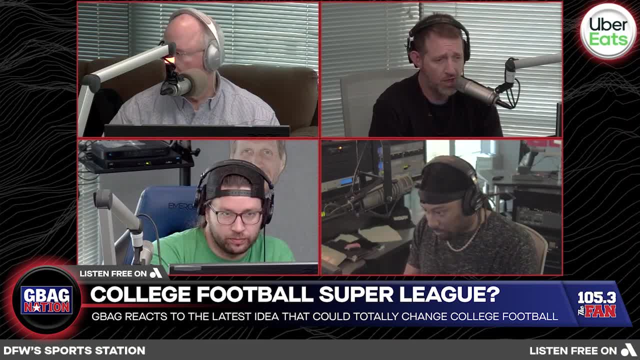 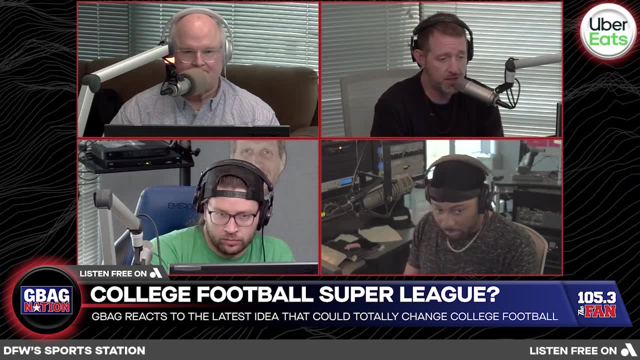 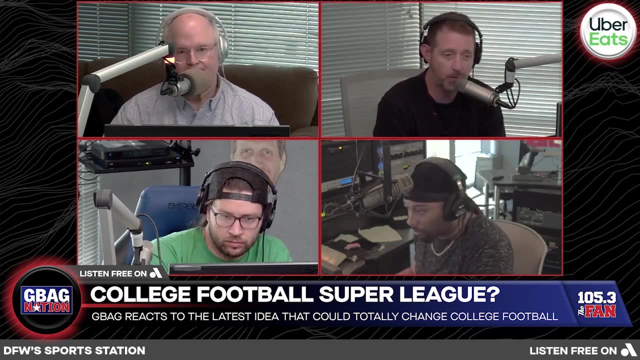 You can go check out the article if you'd like to, But there's 20 different people involved in this group called College Football Tomorrow. They have presidents involved And the main guy quoted says they waited too long to do this. They should have been working towards this a long time ago because they feel like it's probably impossible. 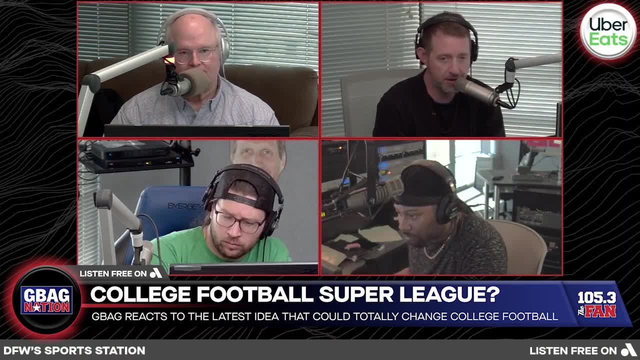 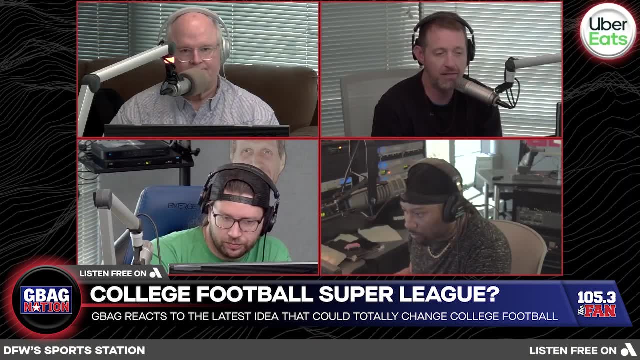 Like a seven-year process, And part of it is letting the old deals expire. But by 2031 would be their goal to bring this to reality. And I was thinking, man, that seems like a long time away. But, Brian, we've become so used to waiting forever for things to change in college football. 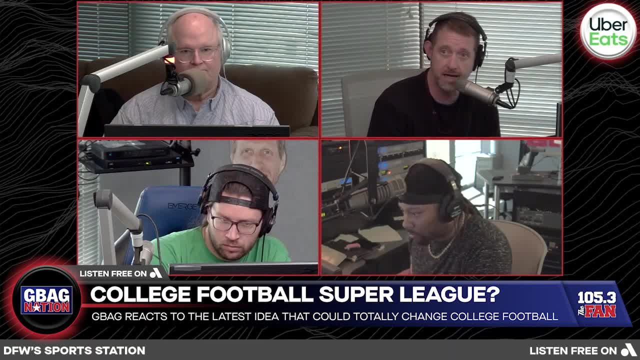 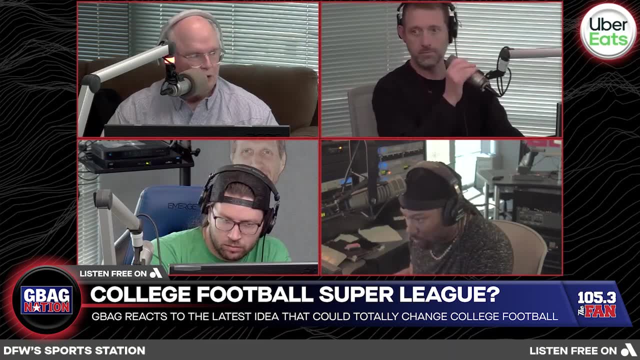 I'm okay with that, As long as they're working towards it. I think that's an exciting piece of what the college football landscape is going to look like. Yeah, I wish they could have come up with it sooner And then been able to hold all the conferences together. 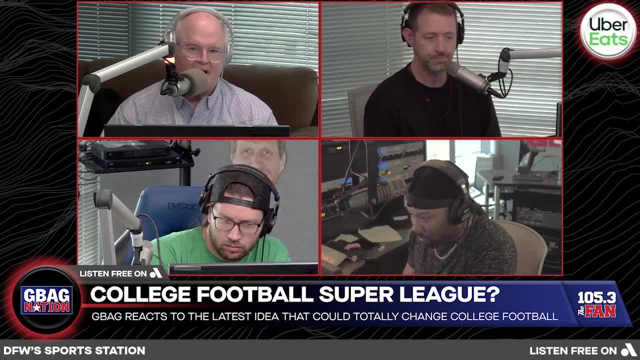 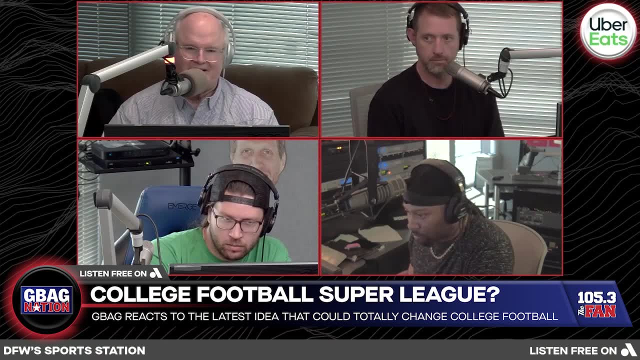 Yeah, You know, We've had now these Pac-12 teams playing in the ACC And Pac-12 teams playing in the Big Ten, And it's a shame because if they could have done this with television, If they could have done it quicker. 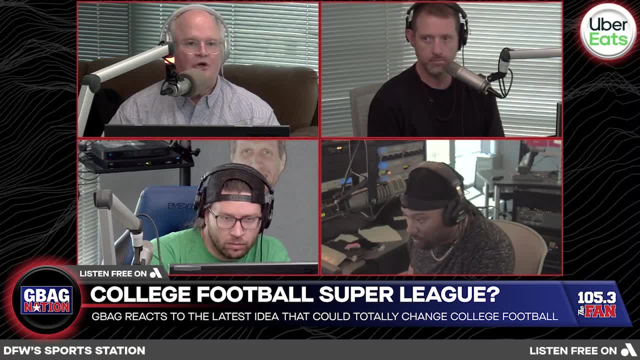 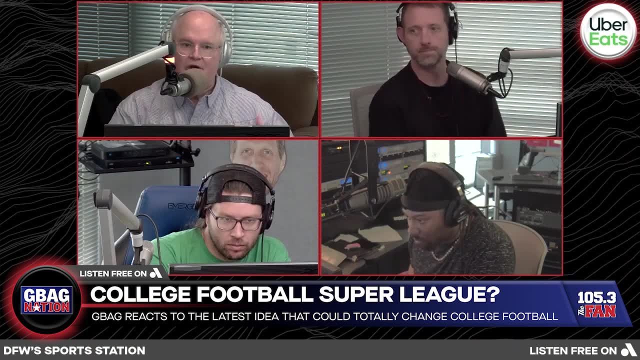 I think you could have saved these conferences Because the money would have been good enough for these teams that are in the Super Conference. They could have funded all the other sports and stuff And kept everybody, so we wouldn't have these, You know. 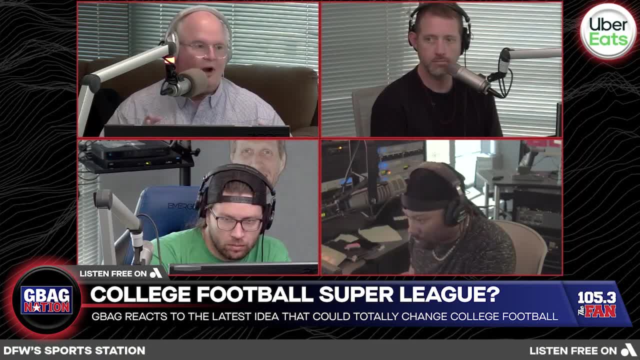 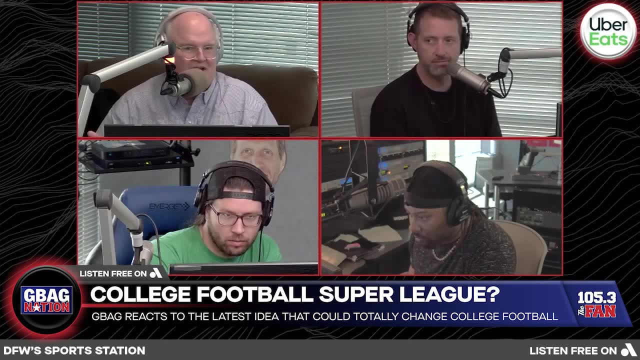 Losing all these rivalries- The football part of it is great, But you're going to lose. You lose rivalries, like in the other sports, And you didn't have to lose that to get this And you didn't have to lose that. 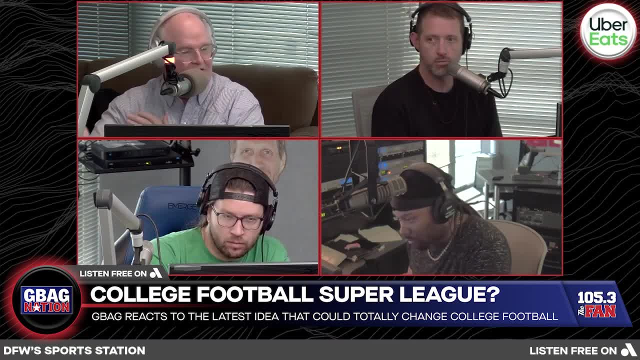 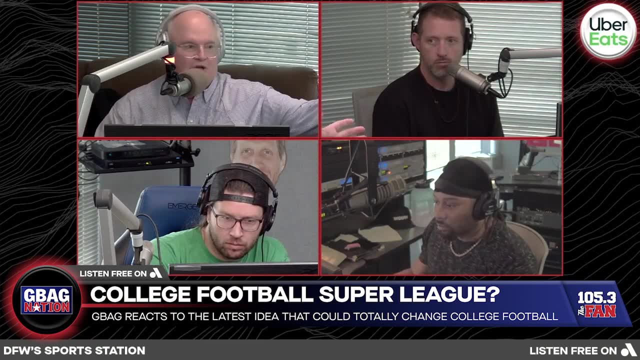 You could have just said: Okay, Michigan, You're in the Super Conference And you know The Michigan, You could stay in the Big Ten And you know, Do all the things you need to do. Or, for example, USC. 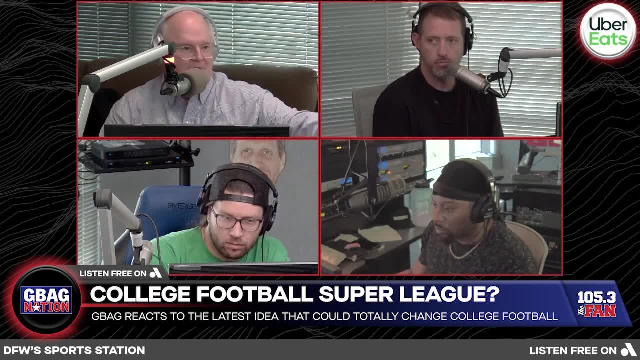 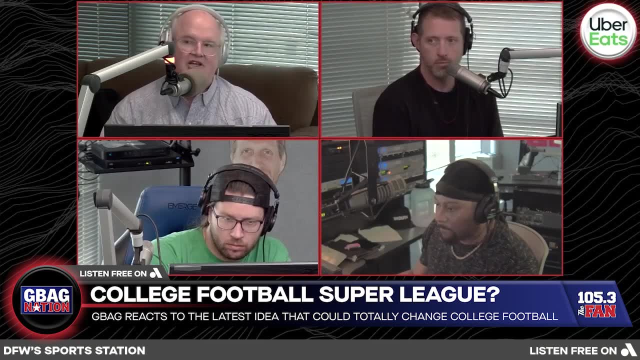 USC. You're in the Super Conference, You get to stay in the Pac-12. And play UCLA And Oregon And all these other teams that you continually play. I think that's where the other sports are going to lose out, Because you're going to lose those rivalries. 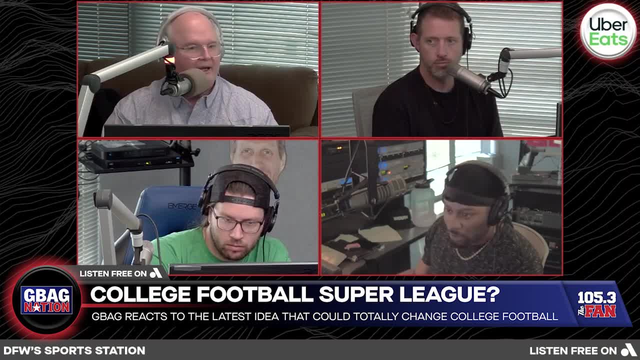 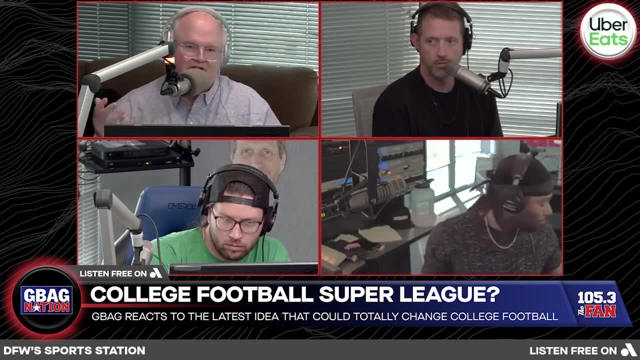 With Stanford having to go now all the way across the country to play North Carolina in a women's sport Or men's sport, Track field, Whatever- It's going to be kind of crazy. They don't have those rivalries anymore. 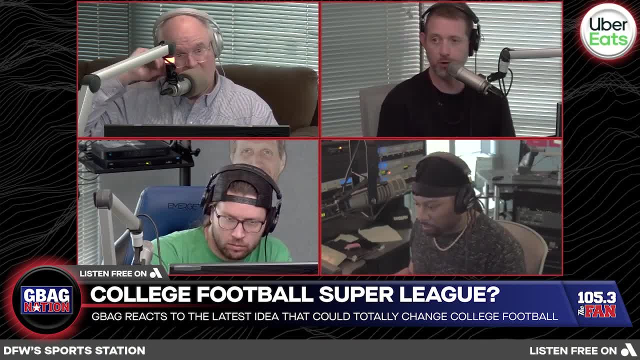 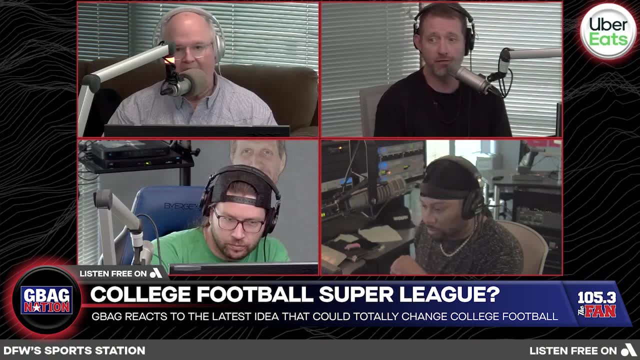 Yeah, It's just weird. You know, The history, The tradition Is something that should have been protected And, You know, Maybe we can start building new history and traditions. But That's a lot of the fun of the sport. 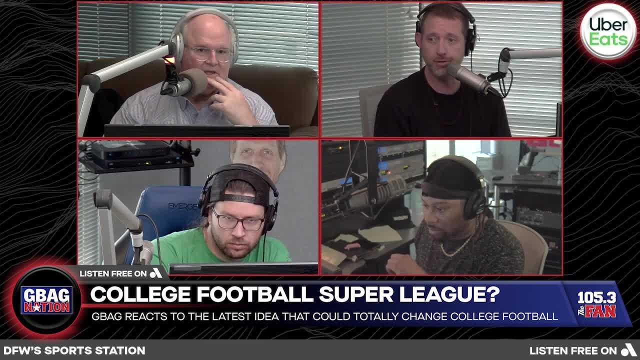 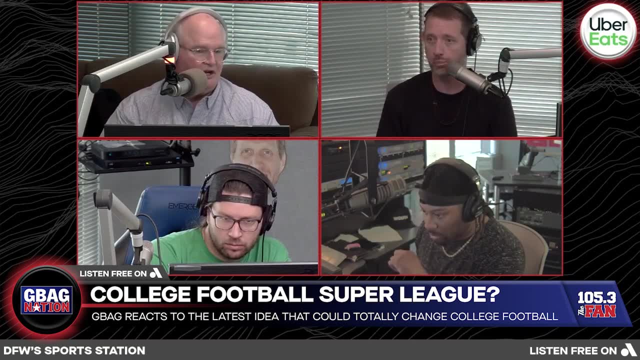 Is the history And being able to drive to most of your rivals. I'm totally okay with LSU playing Michigan and Ohio State. We did that when I was at LSU. We played at Ohio State. We played Notre Dame, You know, Those were fun. 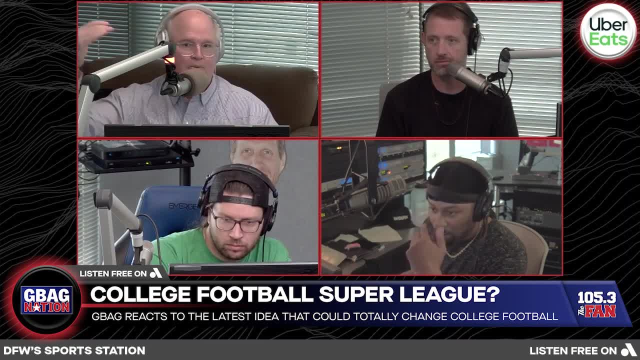 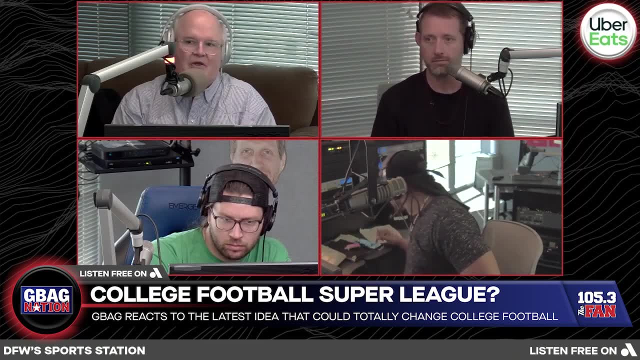 I bet Fun games to be a part of, To go to, like Play at Notre Dame Stadium, Or to play at the SHU, like we did. That part of football I can't. I can't deal with that. It's the other sports. 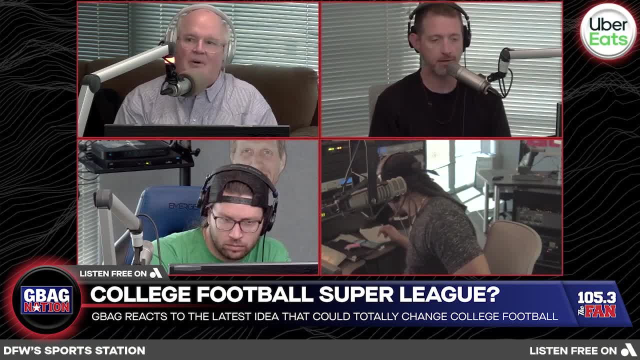 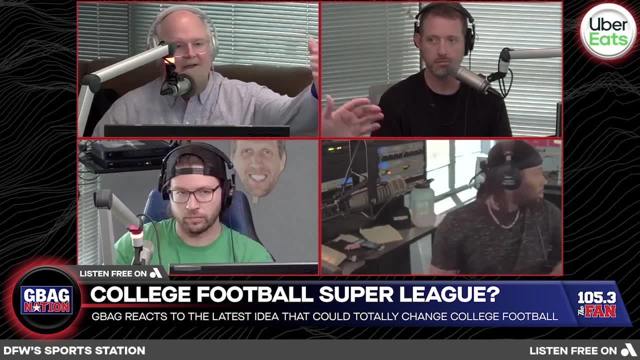 I just don't want to lose those rivalries And I feel like we are. Football rivalries are good, But The fact that we've all We've accepted the fact that Ohio State will play, You know, We'll play Cal. 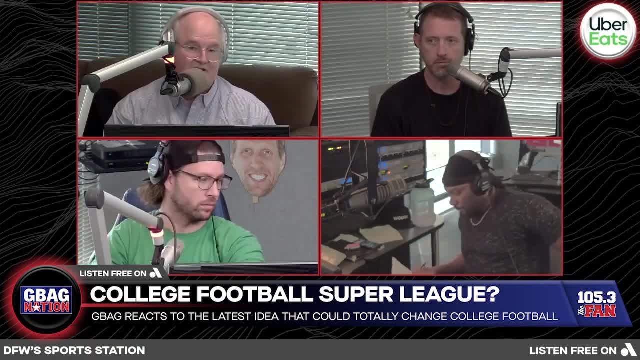 Play USC Or whoever You know. I think that's. I think that's great, But As far as all the other sports, I don't know if that's great. You know that money's going to win, though, Chief, And they want more huge matchups. 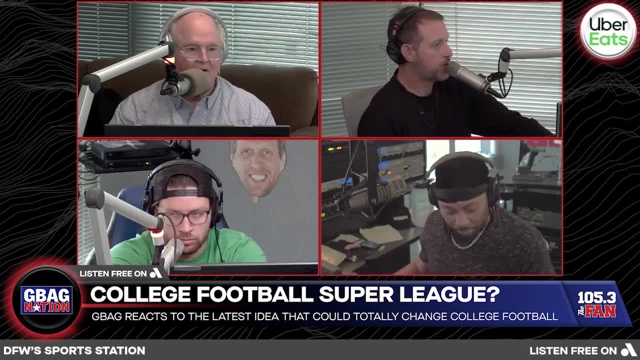 And they're going to get it. There will be- Yeah, That's what they're going to get. There will be less dead weekends. That you can see on Thursday night football- How important it is to have a great game With the most talented players in the sport. 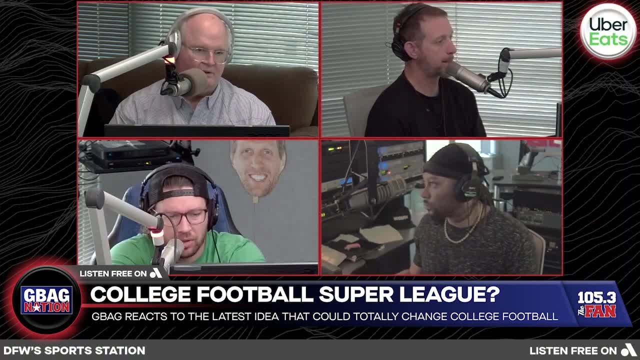 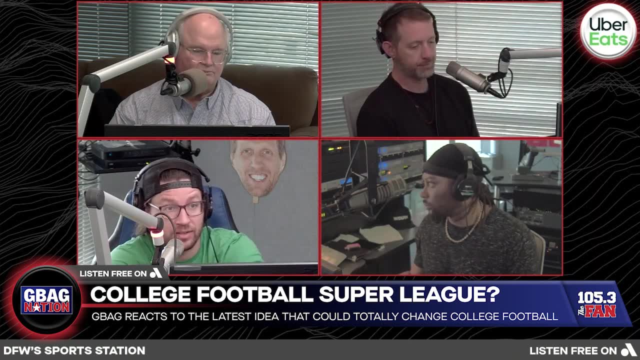 Yeah, Yeah, It's just going to be. There are plenty of weeks in college football Where you're looking around at the slate Going. I mean, Is there one, One game? maybe That is like big, Big money matchup here. 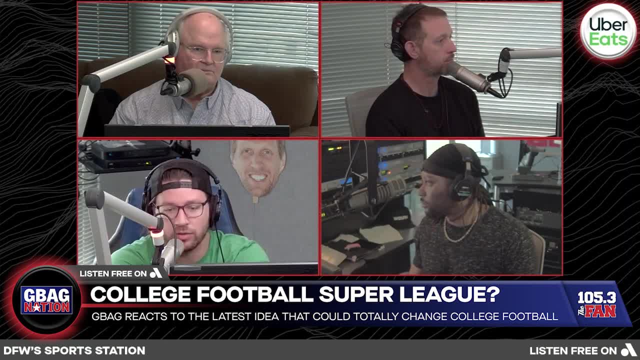 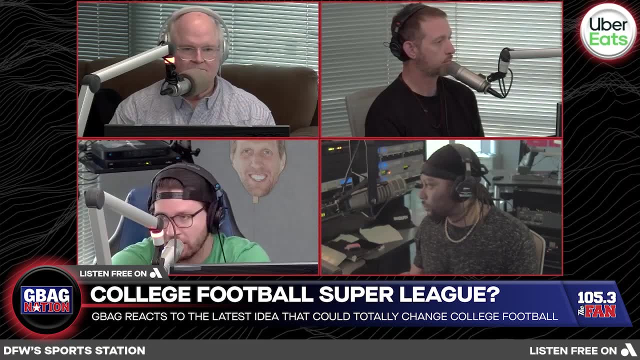 So I'm excited about this. I know the tradition factor Of some things Is going to get Lost In In translation here, Which is a bit of a bummer, But I do think you're getting better matchups. You're getting more high stakes games. 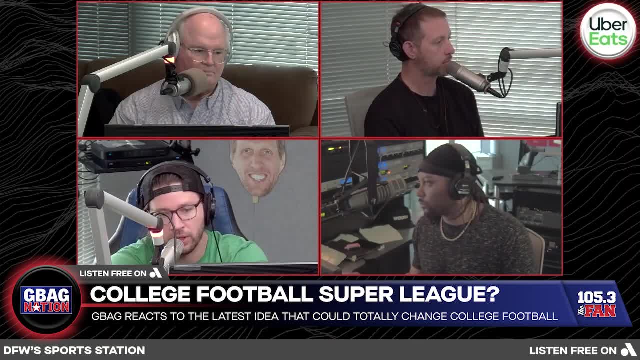 Like when you do You talk about the playoff And all those different things. So, Ultimately, I'm here for all of this And logistically They will figure it out. Yeah, Yeah, And a new history will Will be born. 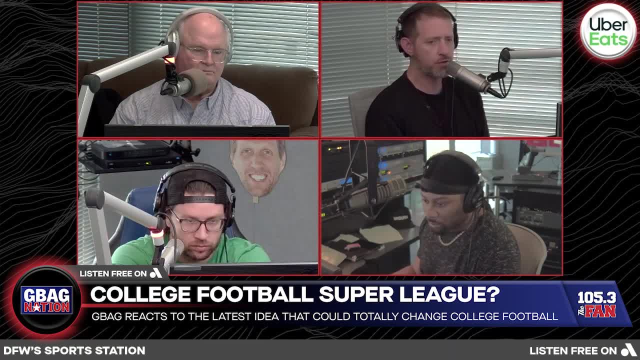 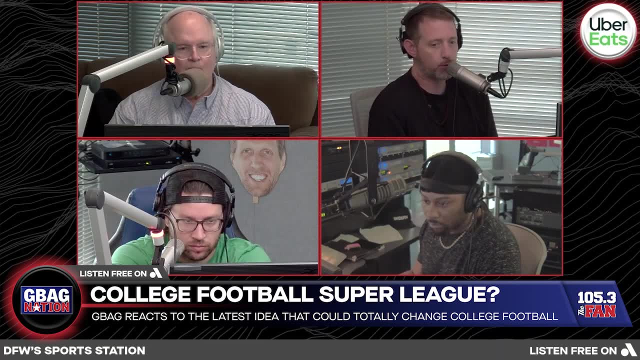 You know Like, For example, In soccer 10.. 12 years ago, Manchester City was an also ran In Manchester United shadow, And now it's become a massive global brand In a very brief period of time Compared to the. 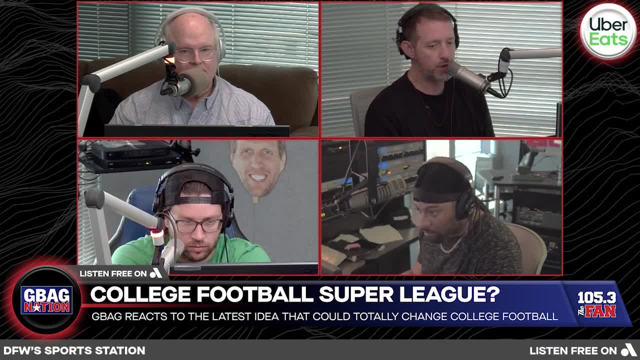 The history of the sport. I think Naturally We kind of resist change And And we don't like it And surely There's value In it- I'm not trivializing, You know- Even losing the Southwest Conference. 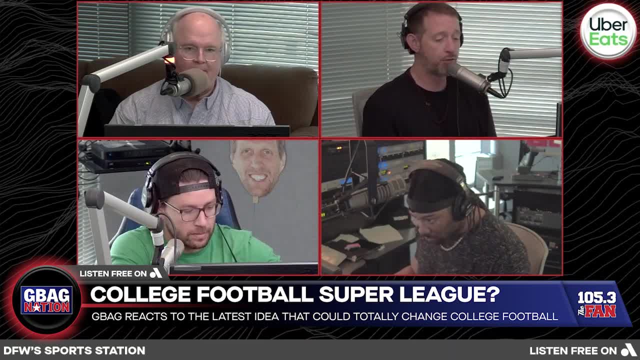 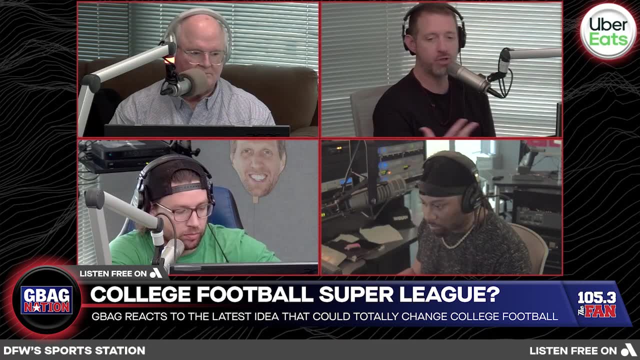 It still sucks All these years later. Yeah, It does. The writer does point out, though, When it comes to the 12 team format, You had commissioners And ADs Trying to hammer that out. They couldn't come to a solution. 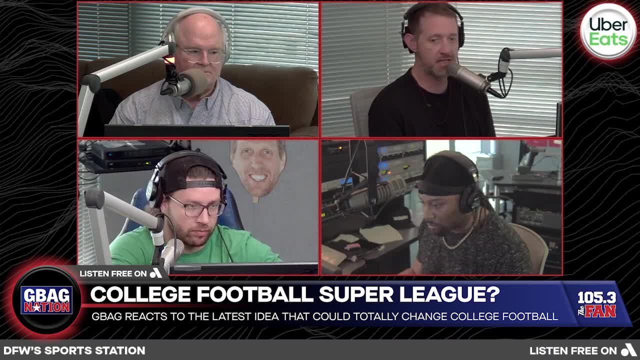 It was like too many chefs in the kitchen Trying to decide on what a menu was going to be, And every time they had a meeting They were like Crap, We're no closer. We got to have another meeting So. 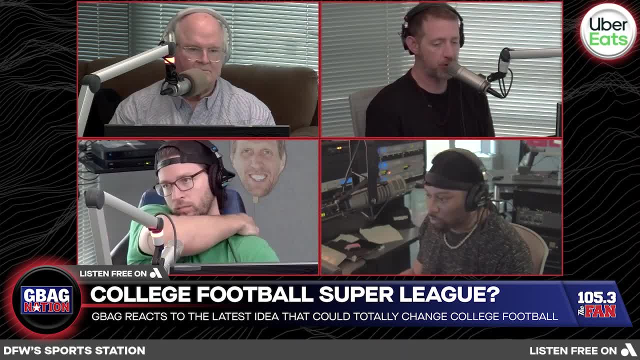 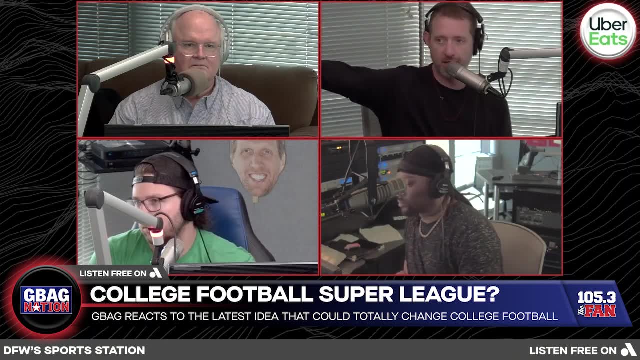 It's taken The college football playoff board of managers, Specifically Mississippi State President Mark Keenum, To get that done And they now see That that process For decision making Inside college football Is vastly superior To the old style. 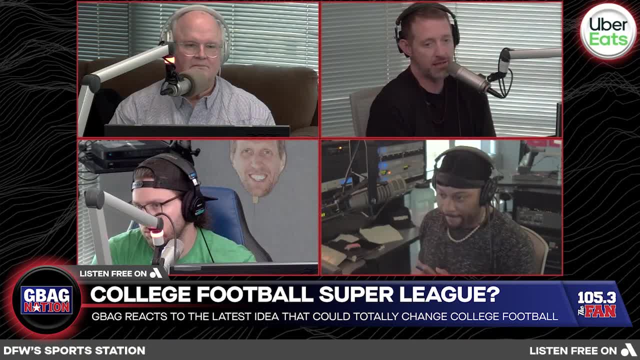 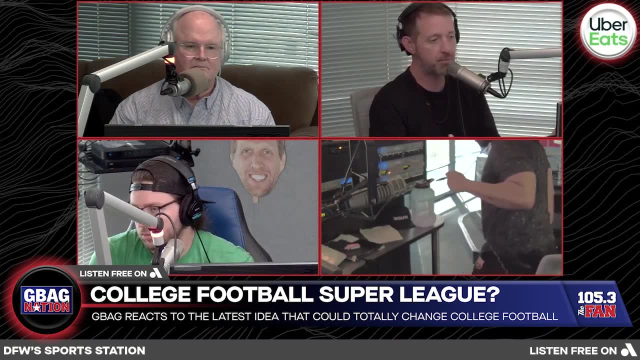 That was just spinning its wheels Trying to come up with this 12 team playoff format. They couldn't get the job done. So, As decisions flow And the logistics Of having meetings, And meetings And committees Decide and vote on things, 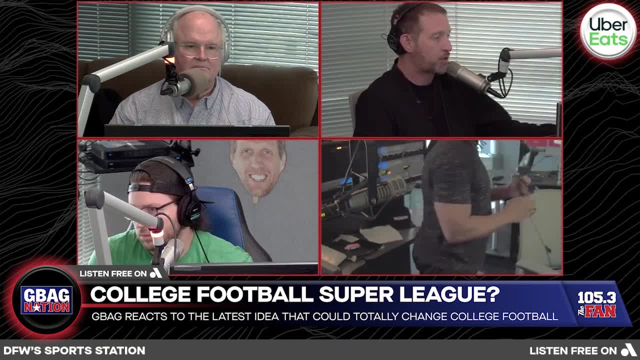 They feel like they've turned over A significant page And maybe college football Doesn't have to move so slow Anymore As a result of it Getting the president, As a result of it Getting the presidents involved. Do you worry about, though? 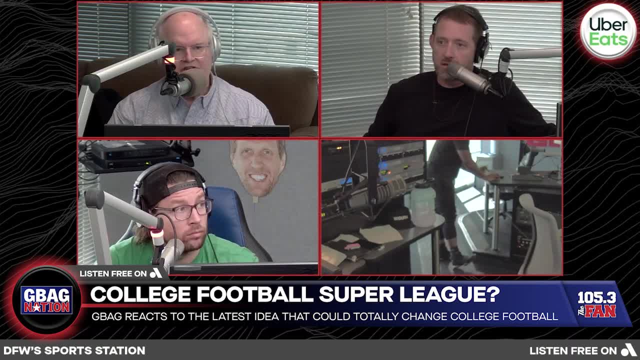 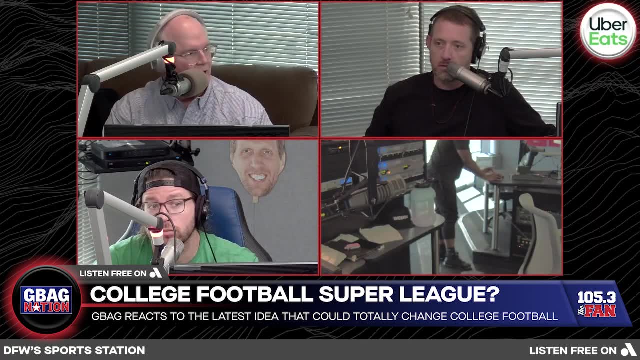 With the Super League That maybe Some of the teams In the Super League, Especially the top teams, Are going to get all the NIL players, All the transfer portal guys. Yeah, Yeah, You think there's going to be. 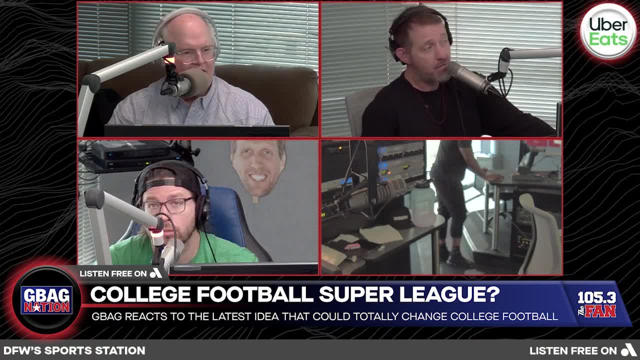 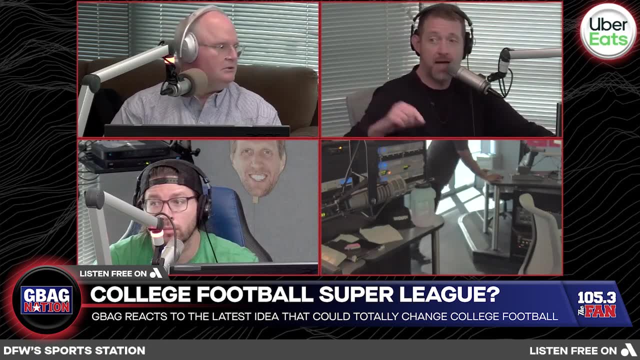 A huge imbalance of players In the Super League That they're all going to end up In the top five Programs. I think You'll have teams That aren't in the top five, Like Man City- Yeah, Who finds a booster? 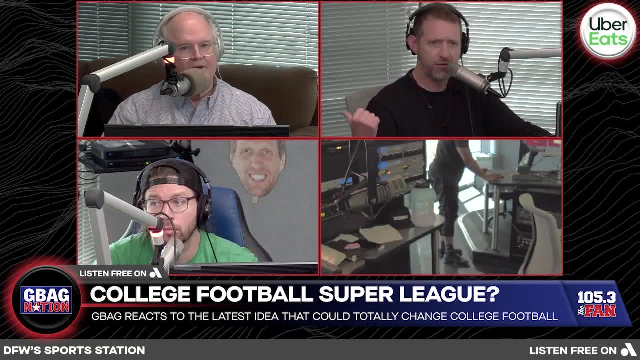 Like: Was it Abramovich That bought it? Yeah, Was it Abramovich? That was Chelsea? It was a different Oil guy, I think he bought Chelsea, Yeah, So like You'll get alumni That come into money. 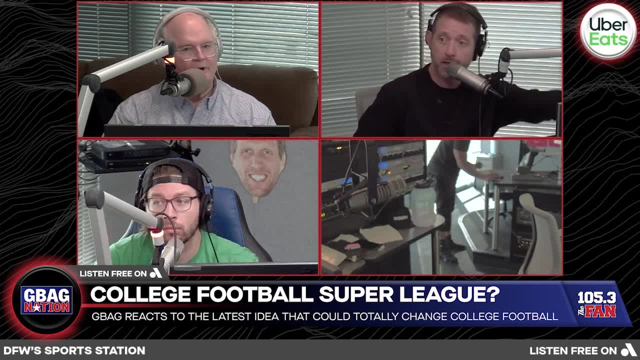 That say, Hey, We're going to make our program great. Like Phil Knight at Oregon Right. He, I think he- went to an Oregon Stanford game In like 1999. Where they won the conference And he was like: 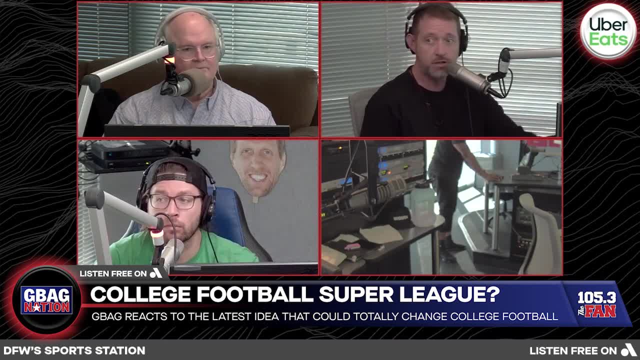 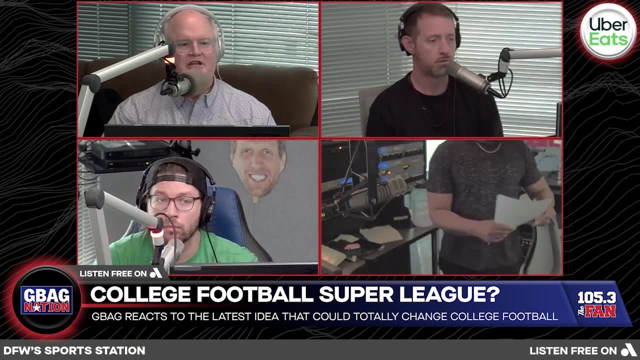 Damn it. I love this And started the process. Next thing, you know, NFL guys are coming out of there. So Right, It's just going to be a. You know, I just wonder if, If the super teams are just 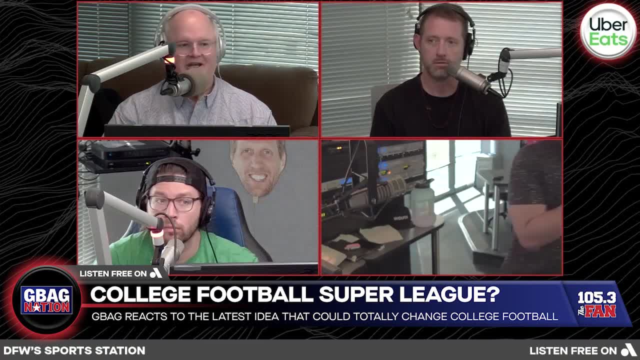 Is there going to be just Maybe Eight to ten Real super teams And everybody else is kind of I mean I would eat more than we have now Is hanging on there, You know, Yeah, I don't know.